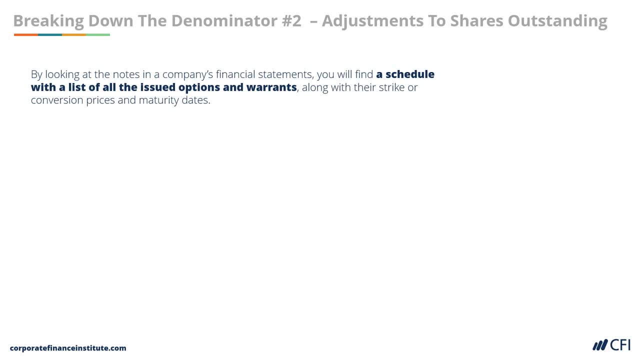 you will find a schedule with a list of all the issued warrants and options, along with their strike price or conversion prices and maturity dates. This is where most of the effort is required. A good financial analyst will recreate a table in Excel with all the details, then compare. 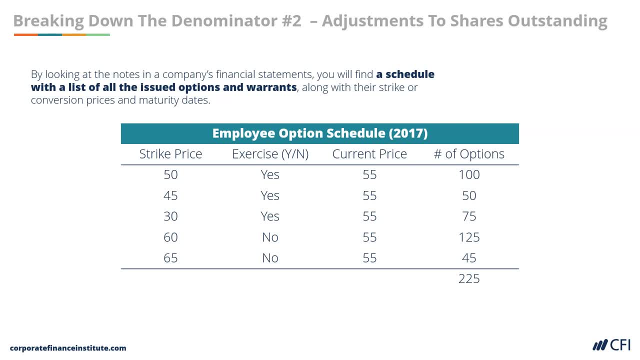 the strike or conversion prices to the current share price or average share price over the period and determine which securities are in the money. In the money refers to an option contract that, if exercised, would be worth some amount of money- Another way to look at. 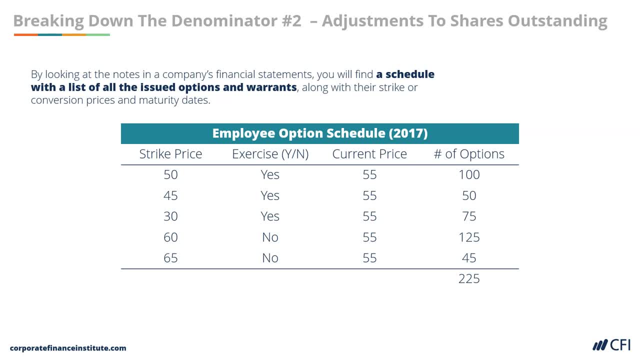 this is to compare the option strike price to the current price of the underlying asset. If the strike price is lower than the underlying asset's price, the option is in the money. The next step is to assume those securities are converted. the company receives the cash. 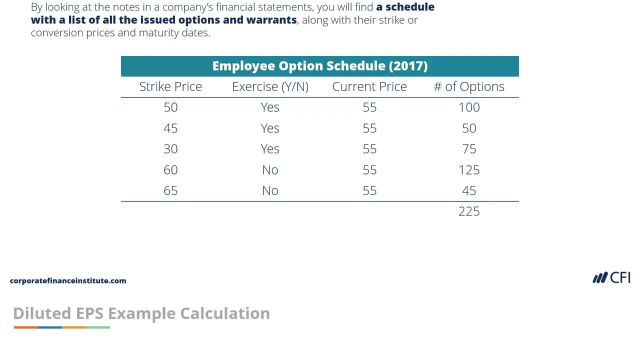 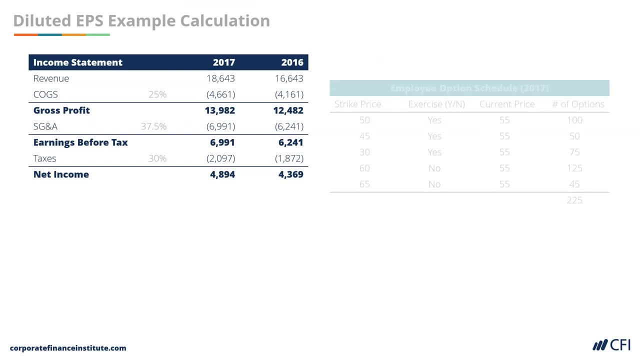 and the number of shares outstanding goes up. Let's take a look at an example of how to calculate diluted earnings per share using an income statement and the option schedule we just looked at. The first number we need to consider is the net income in 2017, which is $4,894. 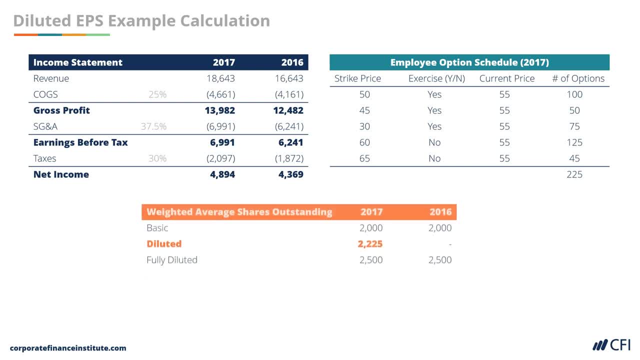 Next, we need to take the number of shares created from the in the money options to reach our number for diluted shares of $2,225.. There are no preferred dividends in this example, so we can divide the net income by the diluted weighted average shares outstanding to get a diluted earnings per share of $2.2. 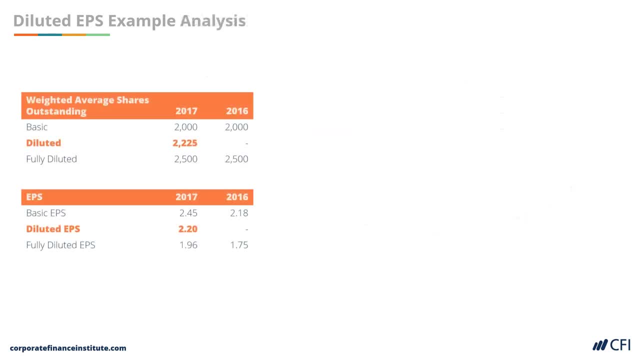 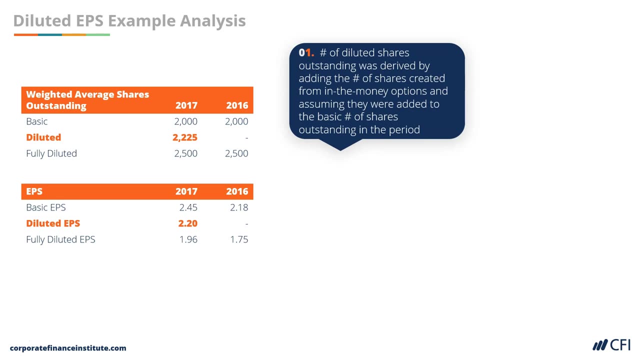 Looking back at this example, we can see that the number of diluted shares outstanding was derived by adding the number of shares that would be created if the in the money options were exercised. We can also compare the three numbers for earnings per share, where we can see that. 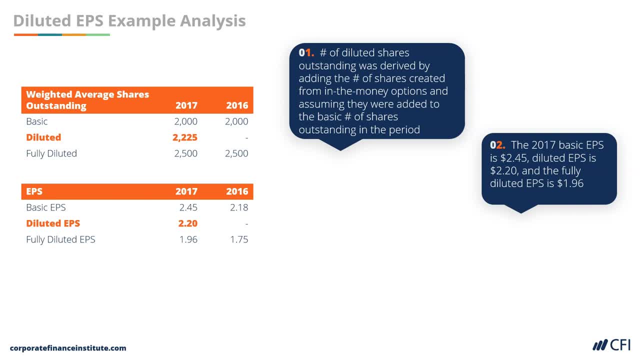 the basic earnings per share is the highest, followed by the diluted earnings per share and then the fully diluted earnings per share. The diluted earnings per share paints the most accurate picture for an investor, while the fully diluted earnings per share shows a more conservative worst case scenario.